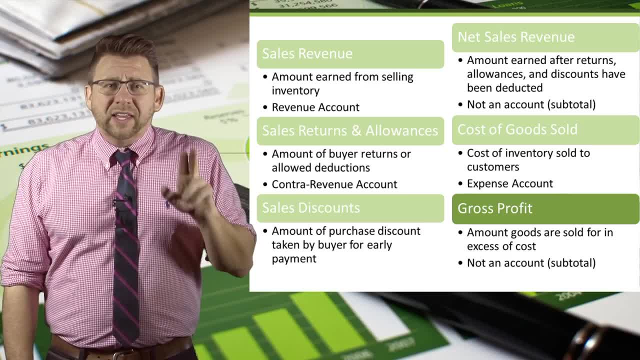 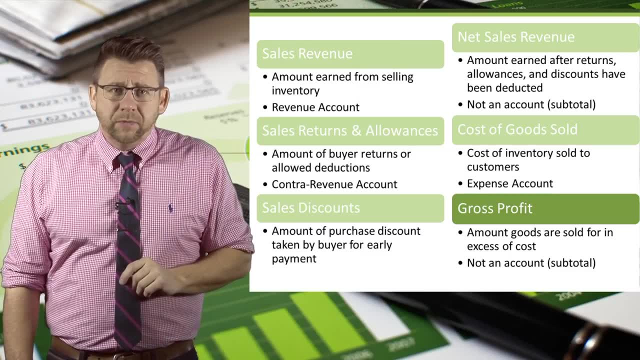 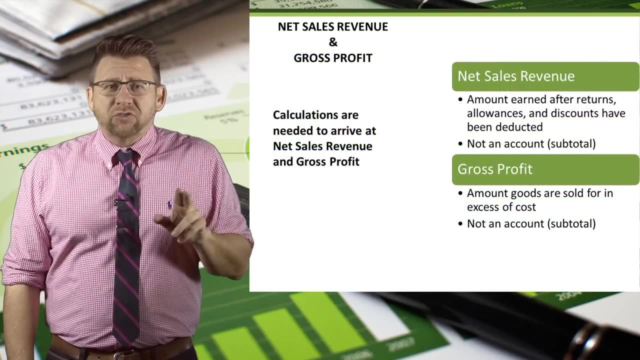 Gross profit is a new term as well. It is the dollar amount goods are sold for, greater than the cost of the goods, It is not an account but rather a sub-total. This is the cost of subtotal- Again. more on that in a minute. Since net sales revenue and gross profit are subtotals, we need to learn how to calculate both. 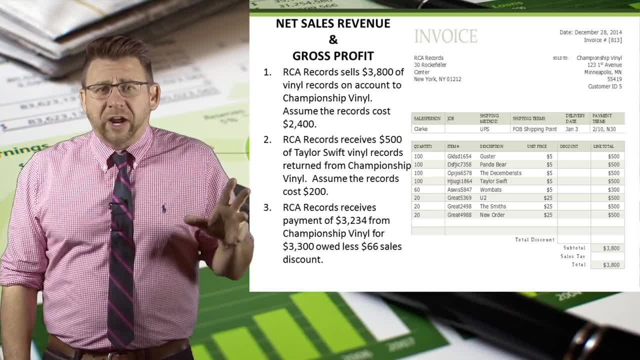 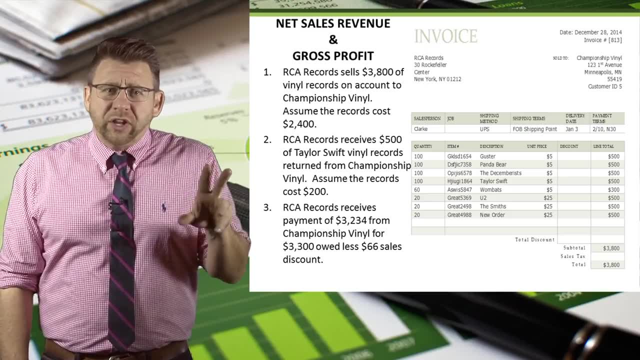 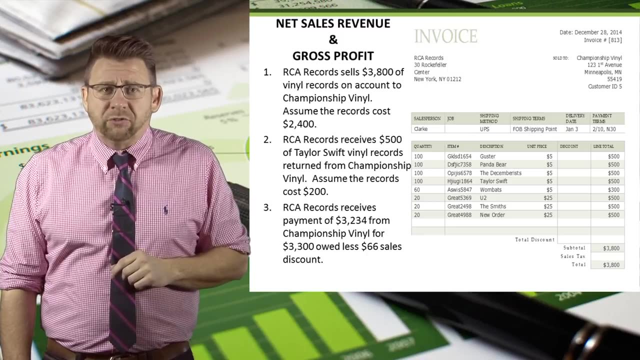 Let's look at the data we used earlier, from the sale of records from RCA Records to Championship Vinyl. Recall that RCA Records sells $3,800 of vinyl records on account to Championship Vinyl. Let's assume that those records cost $2,400.. 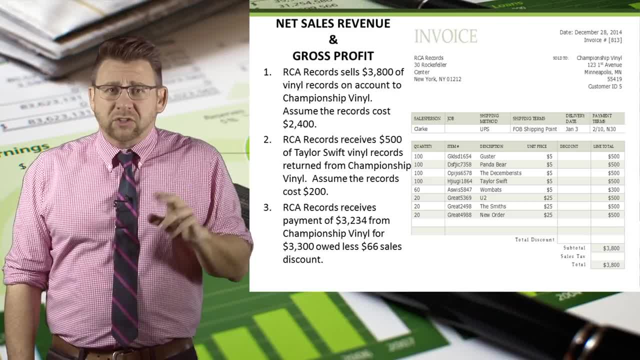 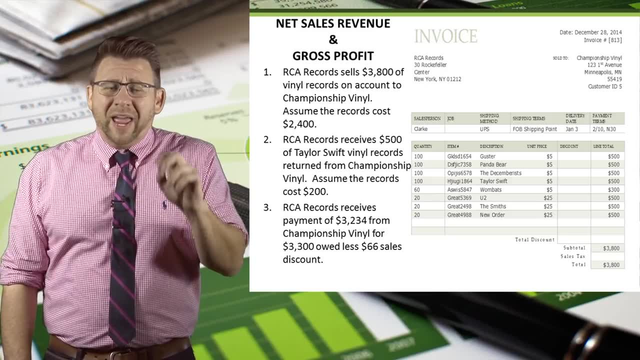 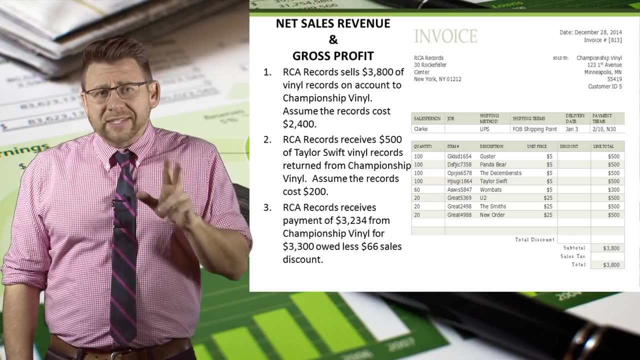 RCA receives a $500 return of the Taylor Swift records. Let's assume that the cost of those records were $200.. RCA Records receives payment of $3,234 from Championship Vinyl, which was the $3,300 owed less the $66 sales discount. 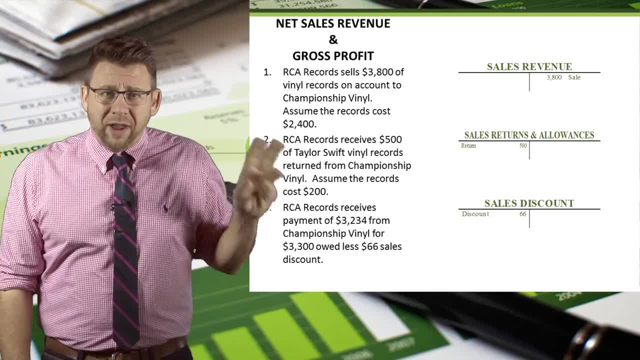 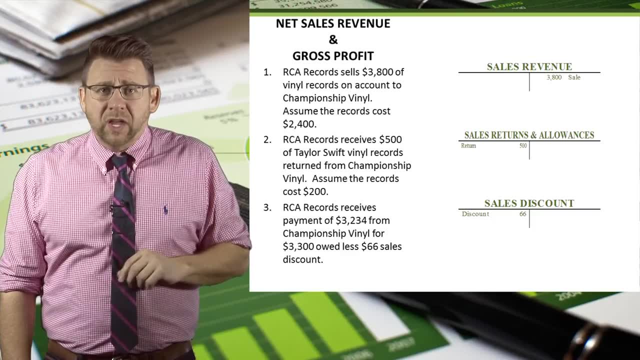 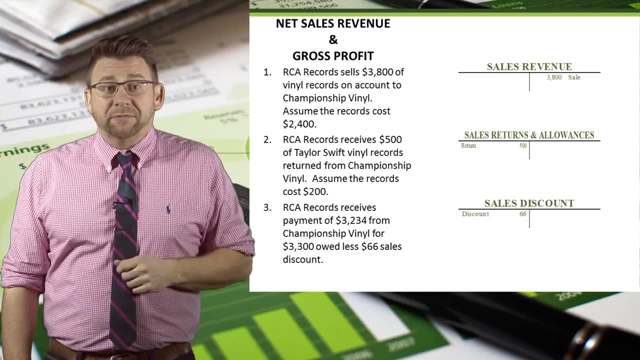 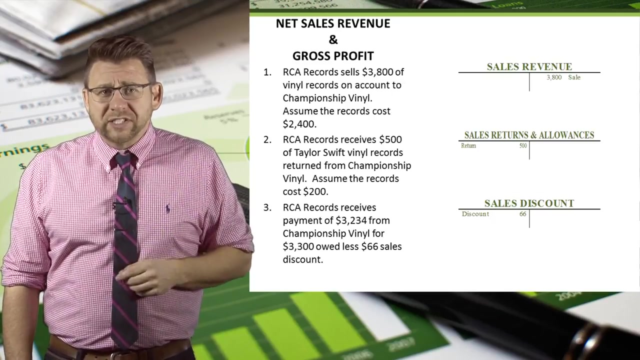 So the T-account looks like this for the revenue and contra-revenue accounts: Sales revenue had a credit balance of $3,800.. Sales returns and allowance has a debit balance of $500 and sales discount has a debit balance of $66.. If you're wondering where those numbers came from, I encourage you to watch the video entitled Perpetual Seller. 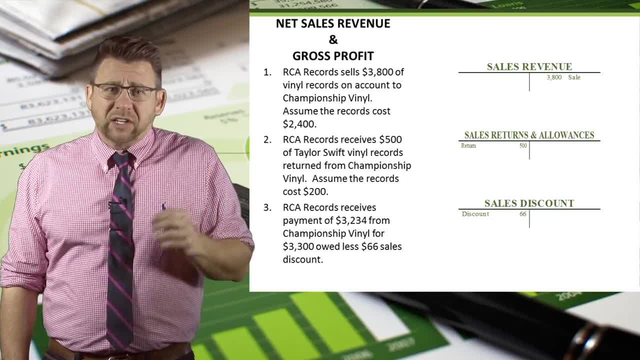 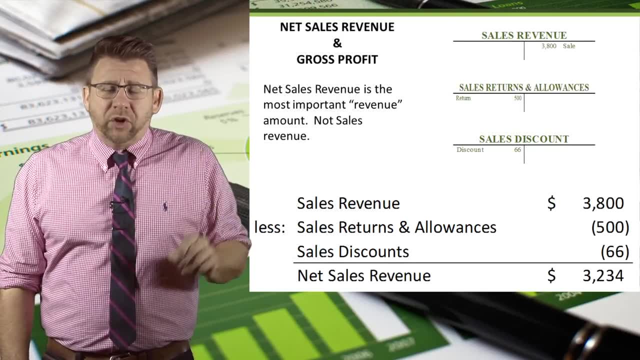 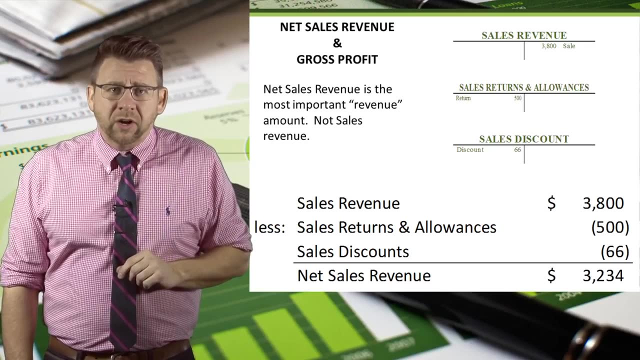 Otherwise, the calculations are the same, regardless of the source of the data. Net sales revenue is calculated as sales revenue minus sales returns and allowances minus sales discount. It is the most important revenue figure because it is the most meaningful to investors and creditors. Here's an example. 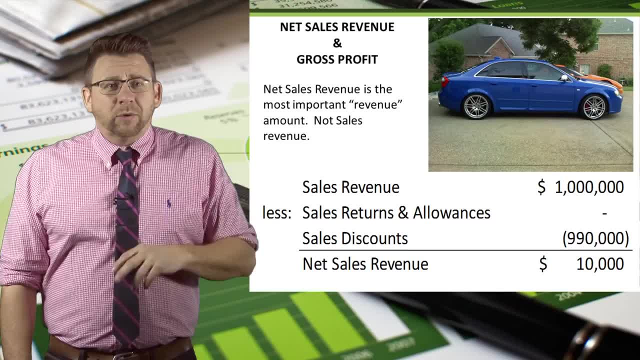 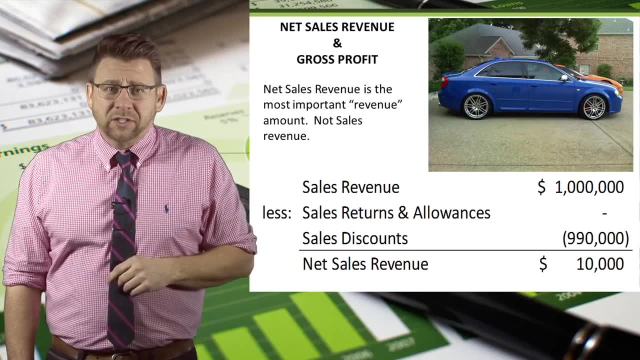 A few years ago I sold my Audi S4. It was a sweet car and, as you can see from the photo, pretty awesome looking, So I figured I'd sell it for $1,000,000.. I mean, look at it, It's cool. 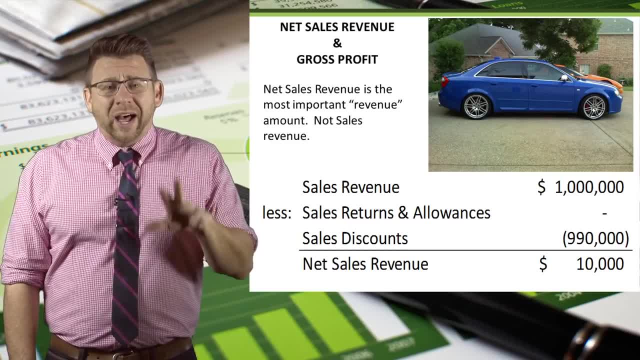 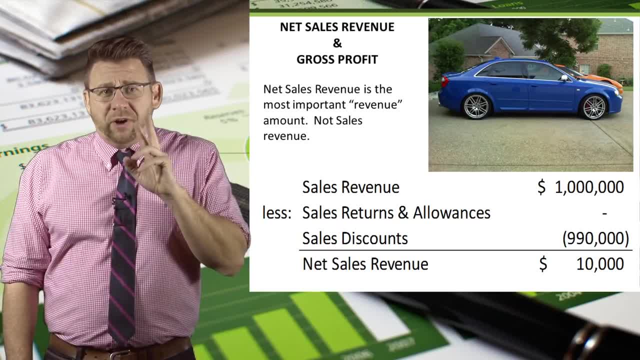 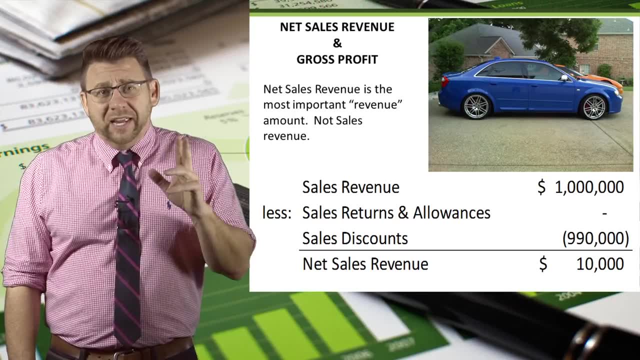 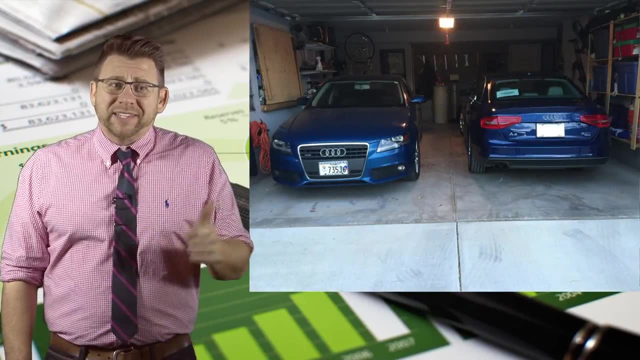 So I offered a $990,000 discount and sold it right away, way. So which amount of revenue provides better information? The million dollars of sales revenue or the $10,000 of net sales revenue? I think you can figure that out. In fact, I like that car so much I replaced it with these two, but that's another story, Now that we know how to calculate net sales. 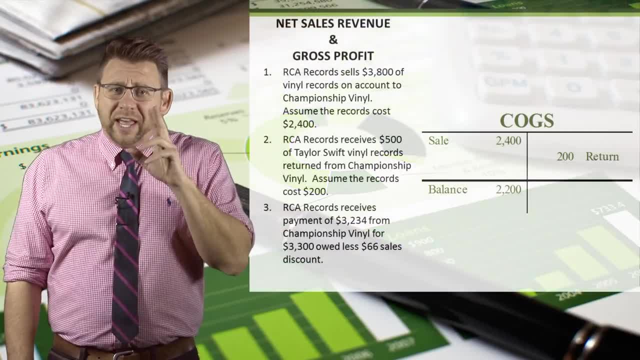 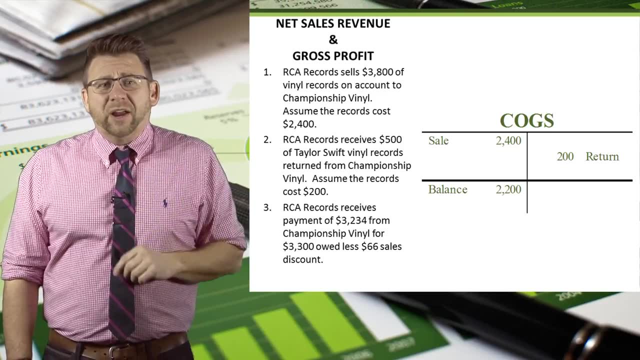 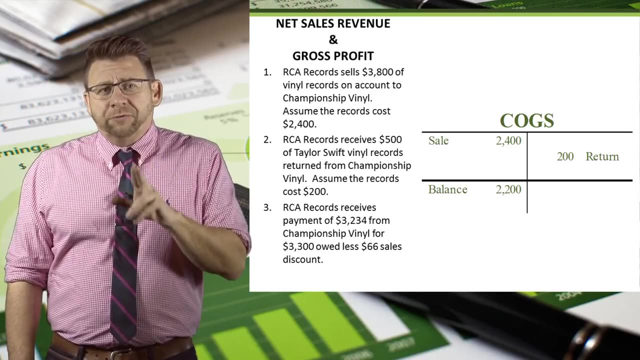 revenue. let's calculate gross profit. In order to calculate gross profit, we need to first figure out the amount of cost of goods sold. When RCA records made the initial sale, cost of goods sold was debited for $2,400, the cost of the records When the Taylor Swift records were returned- cost of 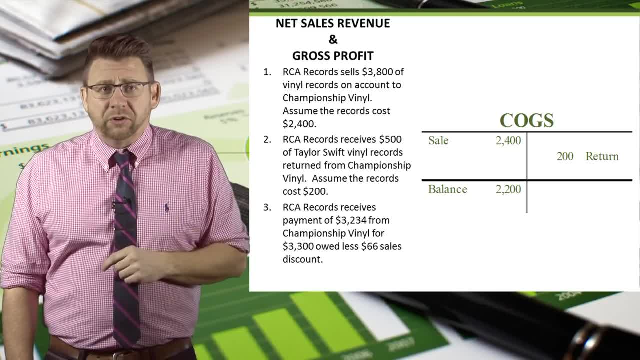 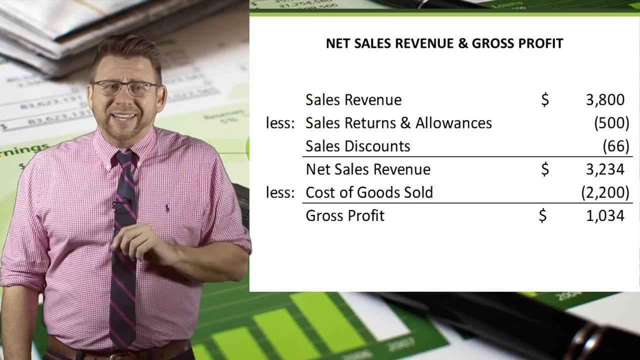 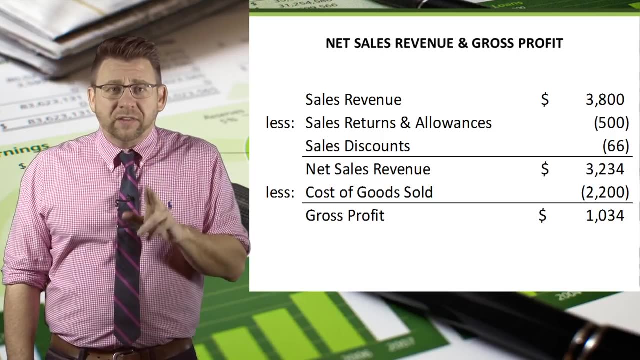 goods sold was reduced by the cost of that inventory of $200.. So the balance in cost of goods sold is $2,200. debit balance Gross profit is the difference between net sales revenue and cost of goods sold. It represents the amount the goods were sold for, greater than their cost. 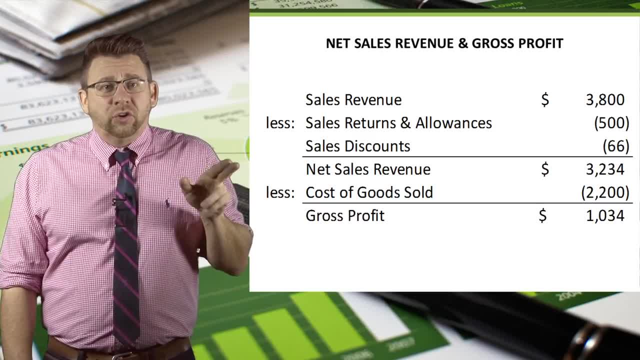 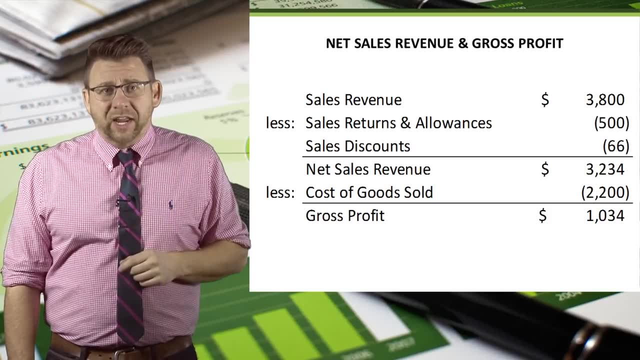 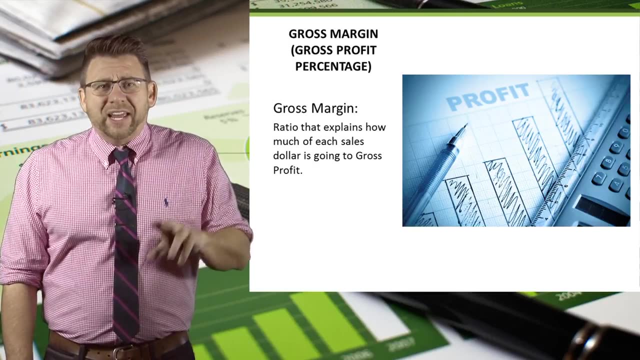 So RCA sold those vinyl records to Championship Vinyl for $1,034 more than they cost RCA records. Gross margin, which is sometimes called the gross profit percentage, is a ratio of gross profit to total sales revenue. Gross margin is the ratio of gross profit to total sales revenue Gross. 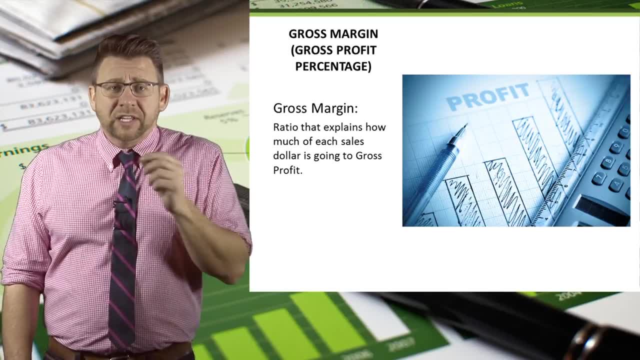 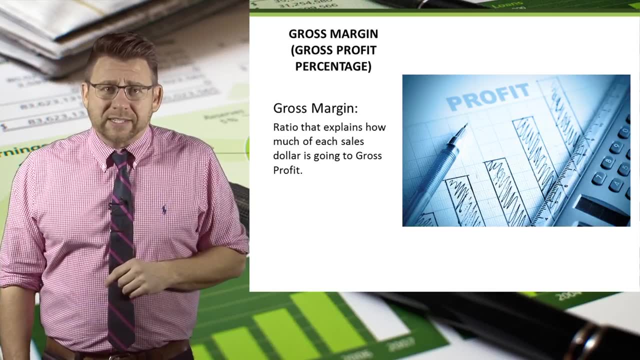 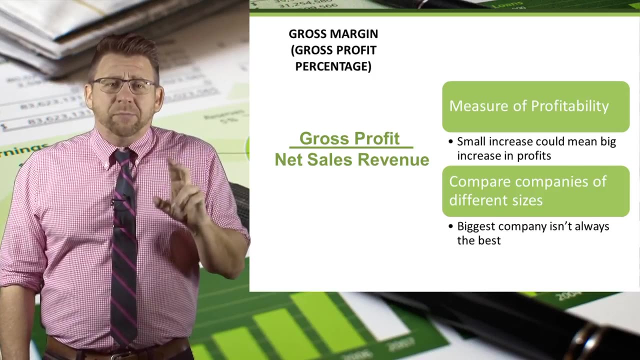 that shows how much of every sales dollars is going to gross profit. This is very helpful for investors and creditors when they compare companies of different sizes. Gross margin is calculated by taking the gross profit in dollars and dividing it by the net sales revenue in dollars. 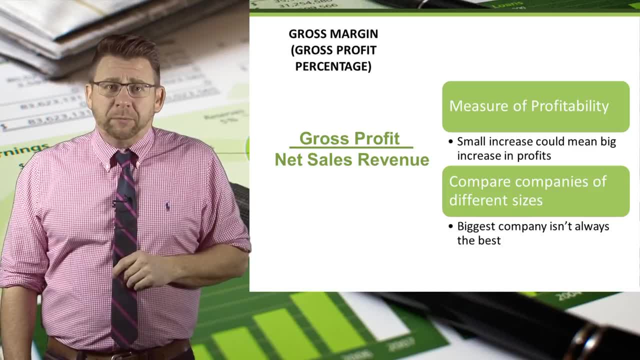 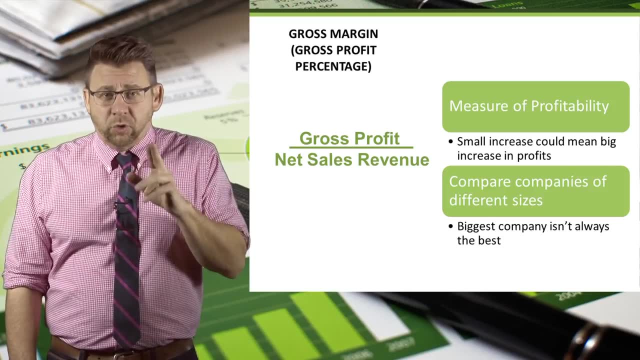 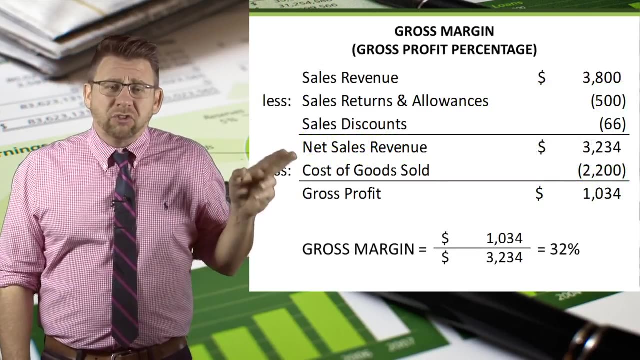 Gross margin is one of the most carefully watched measures of profitability by internal and external users of financial data. A small increase may signal an important rise in income. Conversely, a small decrease may signal trouble For RCA records. the gross margin is 32%. 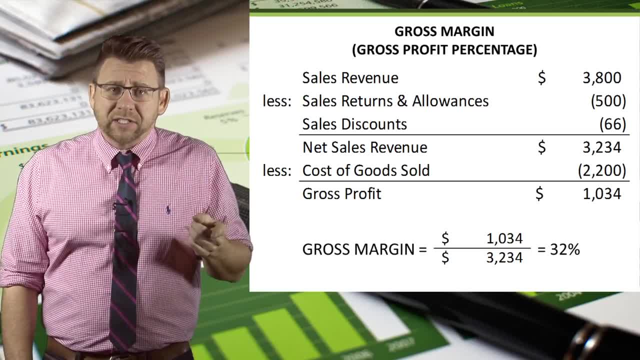 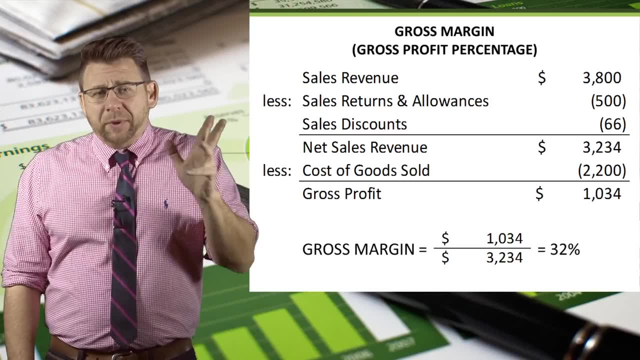 meaning that 32 cents out of every sales dollar is going to gross margin. You'll learn more about how gross margin impacts net income in an upcoming video entitled Multi-Step Income Statement.